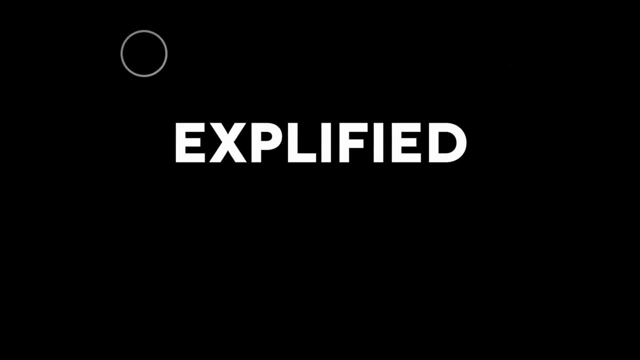 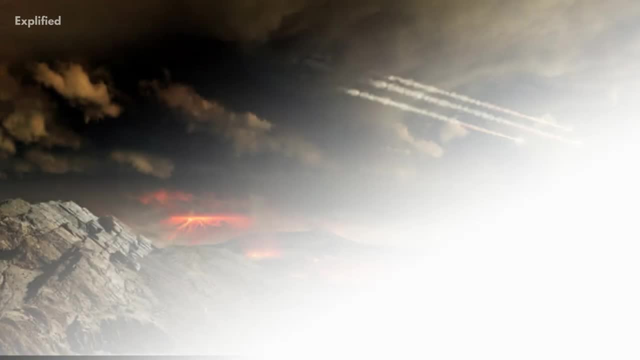 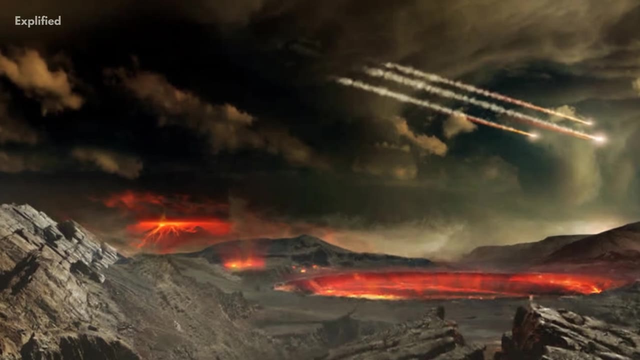 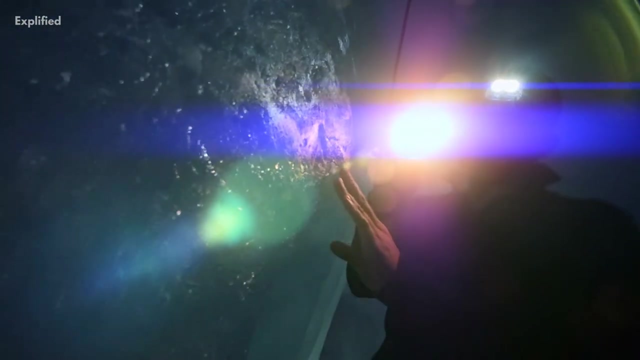 Precambrian period literally means before the Cambrian period. This archaic but still widely used term originally referred to the period of Earth's history preceding the development of the oldest rocks containing recognized fossils. However, geologists have discovered certain difficult-to-find fossils in some Precambrian strata in recent decades. therefore, this period 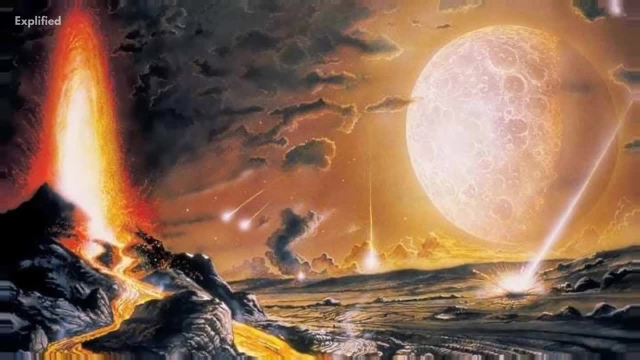 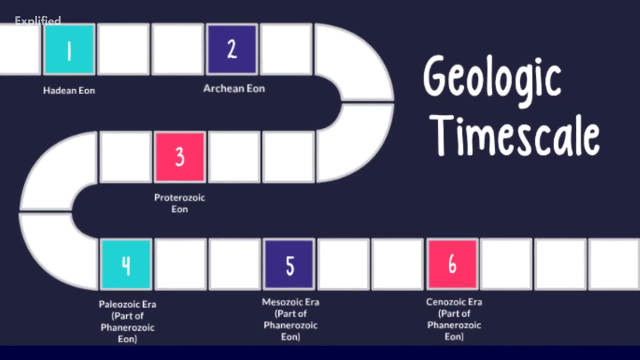 is now known as the Obscure Life or Cryptozoic Eon. The Precambrian period accounts for over 90% of Earth's history. The Hadean, Proterozoic and Archaian eras are the three periods that make up. 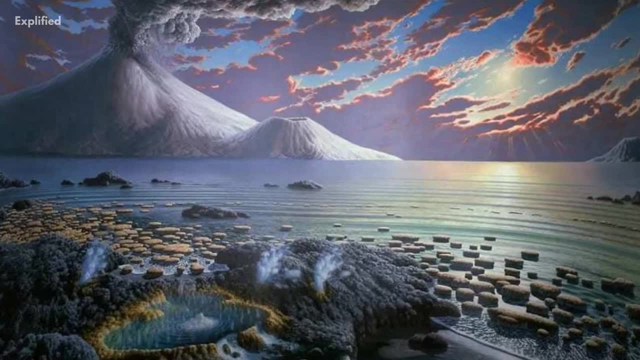 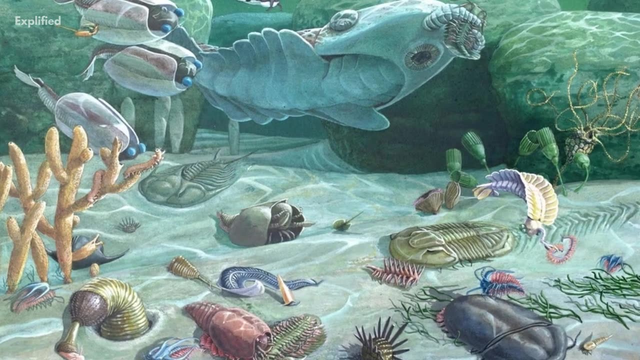 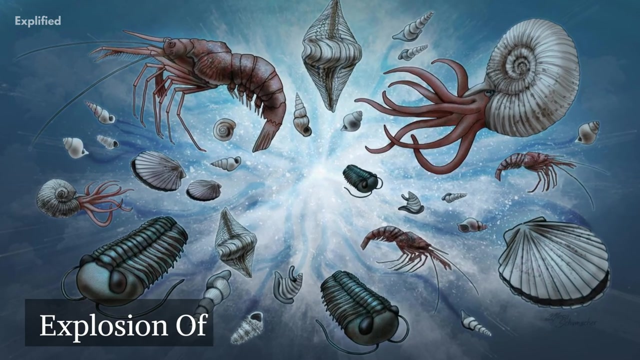 the Precambrian period. The Precambrian era spans the period of geologic time preceding 600 million years ago. The Precambrian period was first characterized as the period preceding the development of life in the Cambrian period. However, it is now known that life on Earth began in the early Archaian and that fossilized species 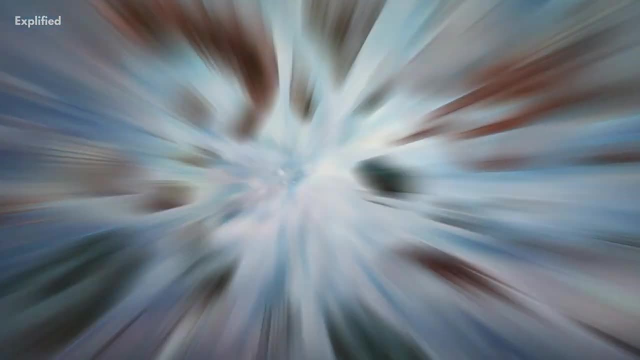 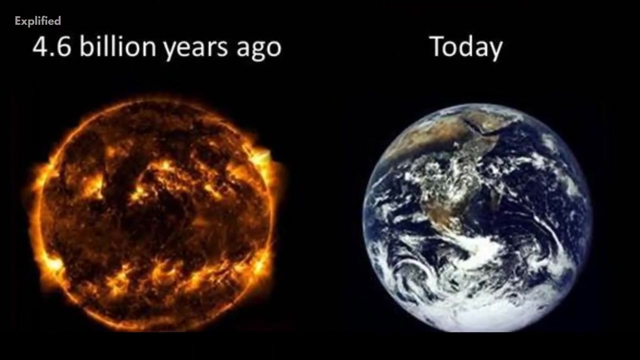 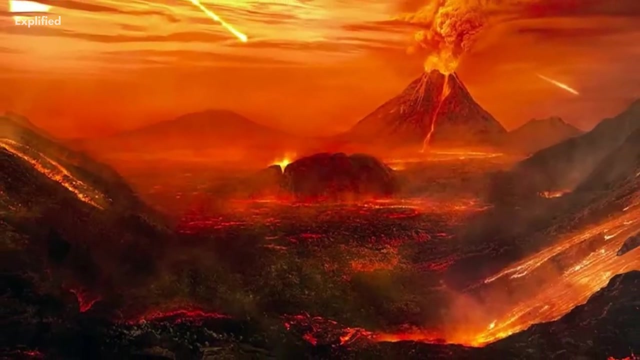 grew in abundance during the Precambrian period. Hadean, or the Hades-like era, was about 4.6 billion years ago. The planet was formed from dust and gas orbiting the sun. During this time, the Earth's surface resembled famous depictions of hell: oceans of liquid rock, boiling sulfur and impact craters. 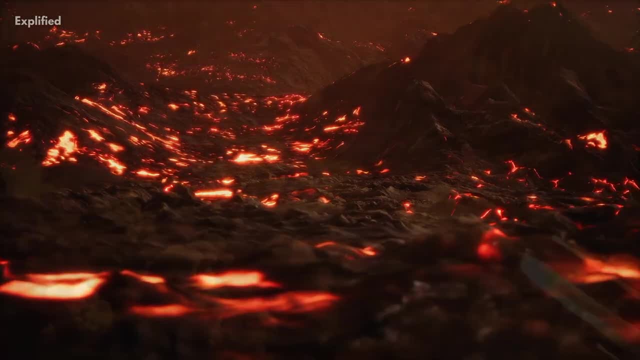 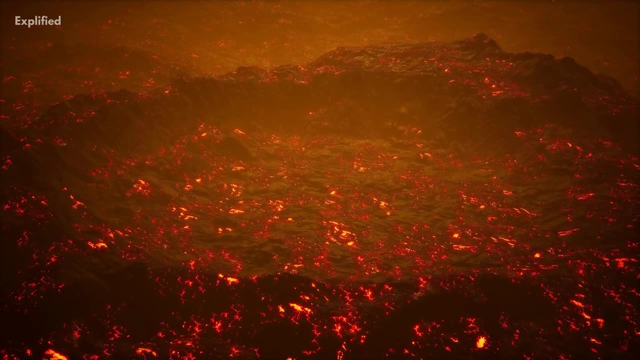 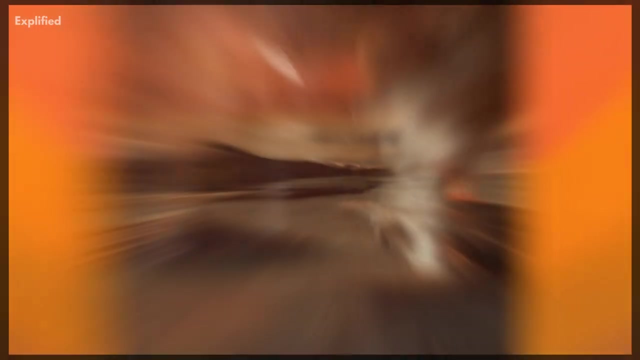 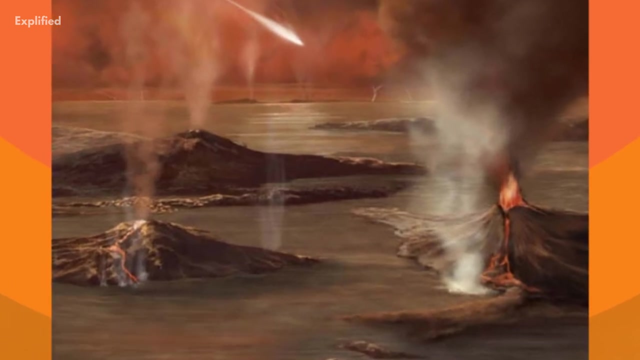 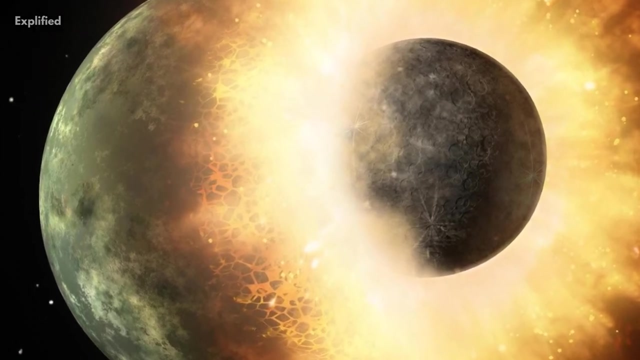 galore. The Earth's surface is covered with dust and grime. However, you can't breathe it because it's made entirely of carbon dioxide and water vapor with traces of nitrogen and odorous sulfur compounds. Some believe that an asteroid the size of Mars collided with the Earth during the start of the Hadean era. Some believe that an asteroid the size of Mars collided with the Earth during the start of the Hadean era. Some believe that an asteroid the size of Mars collided with the Earth during the start of the Hadean era. 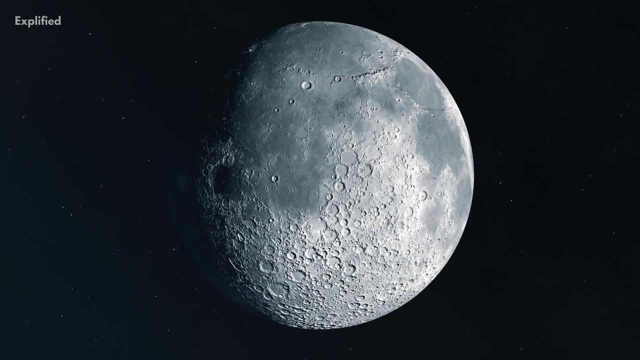 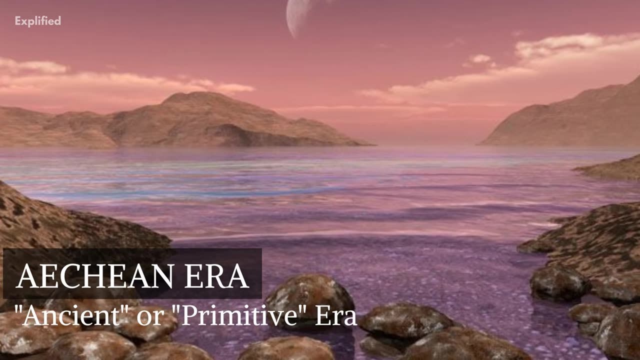 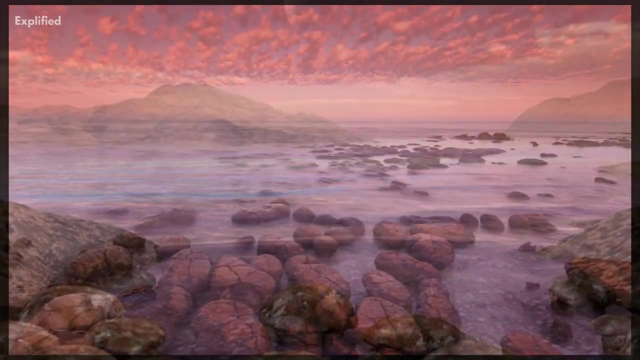 Utterly smashing and melting it and forming the Earth's only natural satellite moon. as a result of the process, Archaian era is also known as ancient or primitive era. This age begins almost a billion years after the Earth's origin, and things have changed dramatically. Everything has mostly cooled down.